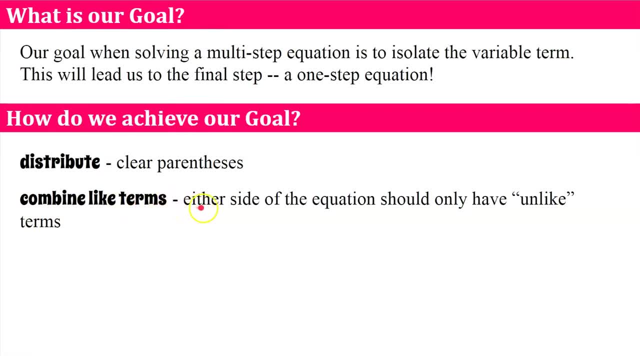 are like terms that can be combined. So we'll examine either side of the equation and each side should have of the equal sign, should have only unlike terms. And then we're going to look to isolate the variable term by adding or subtracting a constant term. So these are three methods. I'm 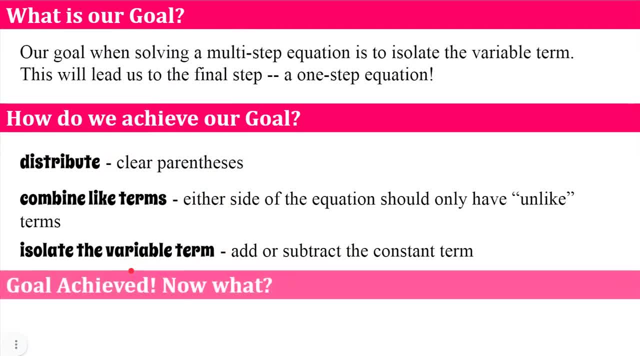 going to show you today in the multi-step process. Now our goal is achieved. Now what We are going to clear the coefficient. We're going to multiply or divide both sides of the equation by the coefficient, which is when we get to our one step. 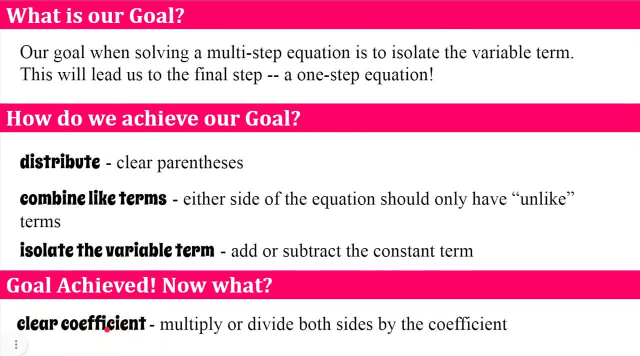 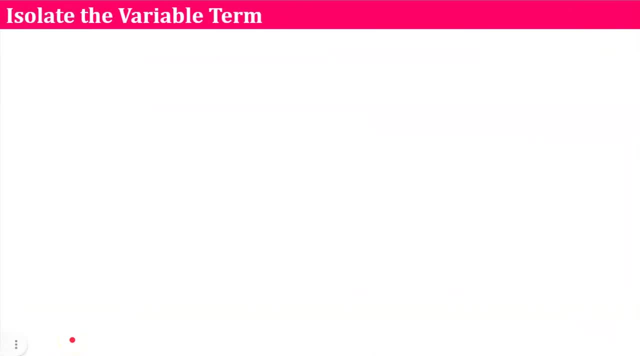 So the previous video talked about using inverse operations, and what you were doing was clearing the coefficient to solve for the variable. Let's try one. The first example I'm going to show you is one that's referring to as isolating the variable term. 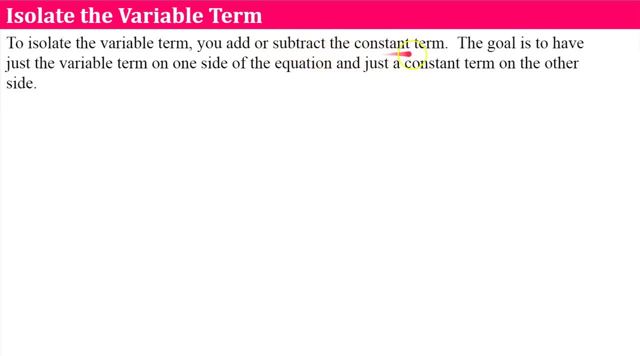 To isolate the variable term. we're going to add or subtract the constant term. The goal is to have just the variable term on one side of the equation and just the constant term on the other side. So here we have an equation: 11x plus 4 equals 48. And remember, we're solving 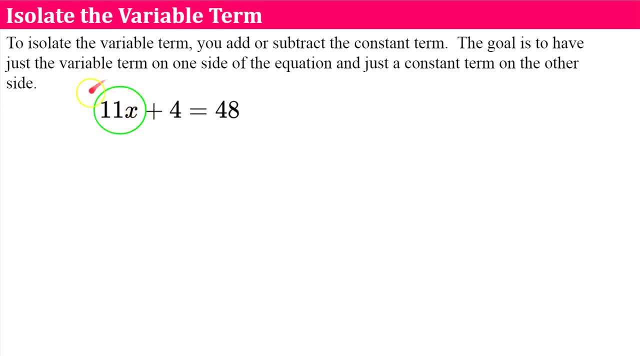 for x. So the first thing I want to do is identify where that variable term is. This is my unknown. This is what I need to get all by itself. So there we get this term: Isolate the variable term. That's our goal. We want to get this 11x all by itself on one side of the equal sign. 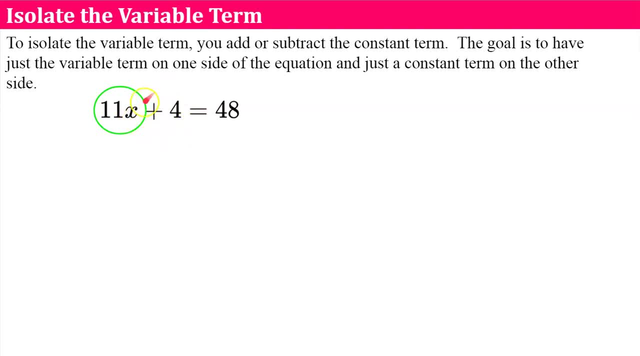 So I look at what's happening to the variable term and it's being added by 4.. Well, the inverse of that is to subtract 4.. If we subtract 4 from the left, we must subtract 4 from the right side. 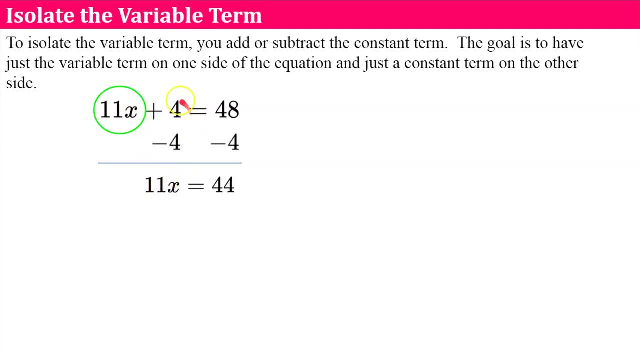 So let's subtract 4, leaves us the 11x, because this is 0.. 48 subtract 4 is 44.. Now, this is what we were looking at in our previous video. This is what we call a one step equation. 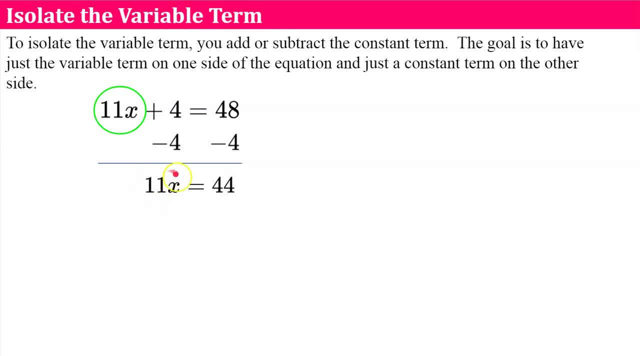 So now we want to clear this coefficient. The 11 that comes before the variable is what we call a coefficient, And again we want to know just what x is equal to. So what is happening to x? It's being multiplied by 11.. The inverse of multiply by 11 is to divide by 11.. If I divide the left, 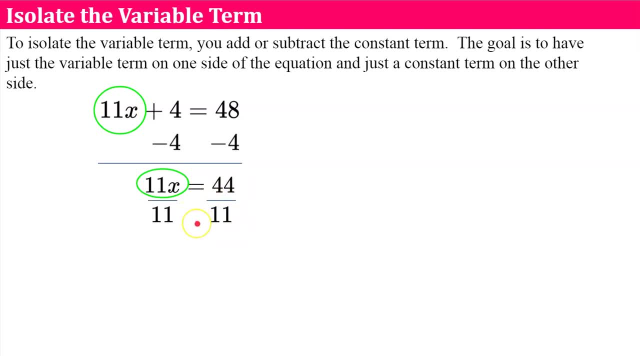 side by 11, I must divide the right side by 11.. Now we can simplify: 11 divided by 11 is 1,, giving me 1.6.. 1x or just x, and 44 divided by 11 is 4.. So I have a solution: of x equals 4.. 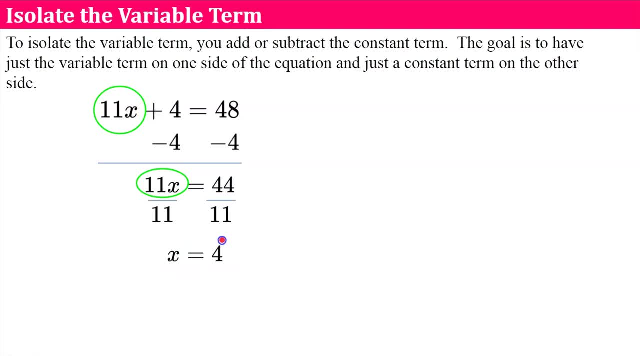 If you remember back to when I previewed the lesson, I asked you to think about one question: How can you be sure that you've correctly solved the equation? Here's how We're going to check. So we're going to plug in. We're going to take this x equals 4 and replace the variable x in the original equation. 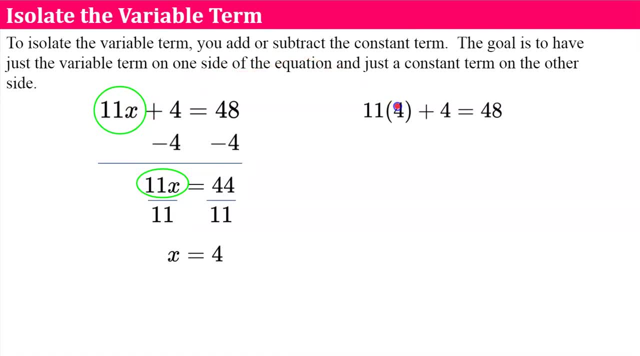 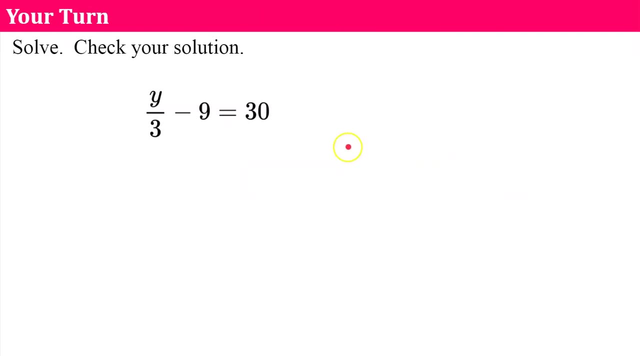 value 4.. And if we did everything correctly, it's going to check 11 times. 4 is 44 plus 4 is 48. And it checks Your turn. I would like you to try. Please pause Solve, Check your solution. Come back when you're done. 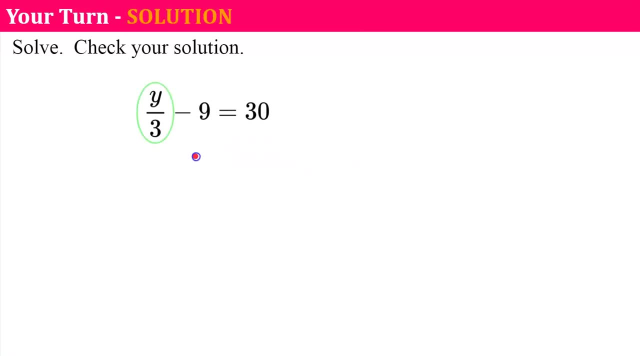 Welcome back. So the first thing we want to do is identify our variable term. Here it is: It's being subtracted by 9.. Instead of subtract 9, we're going to do the inverse and add 9 to both sides of the equation. We'll simplify: Negative 9 and 9 are opposites and equal 0.. 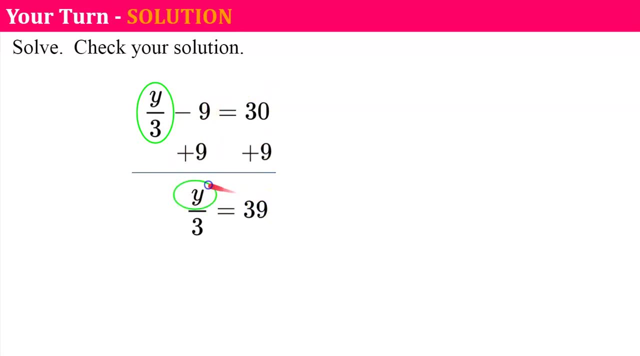 30 plus 9 is 39.. Once again, here's my variable. What's happening to my variable? It's being divided by 3.. The inverse of divide by 3 is to multiply by 3.. I'm going to multiply both sides of the equation by 3.. 3 divided by 3 is 1, leaving me just my. 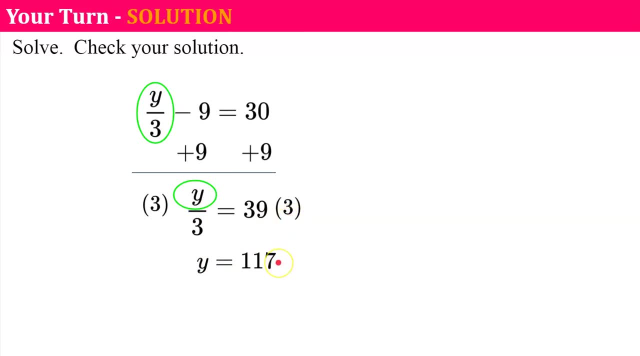 variable on the left, And 39 times 3 is 117.. Now, going back to that essential question: how can I be sure that I have the correct solution? I'm going to check, So I'm going to go back to my original equation and replace y with 117.. This is what it would look like. 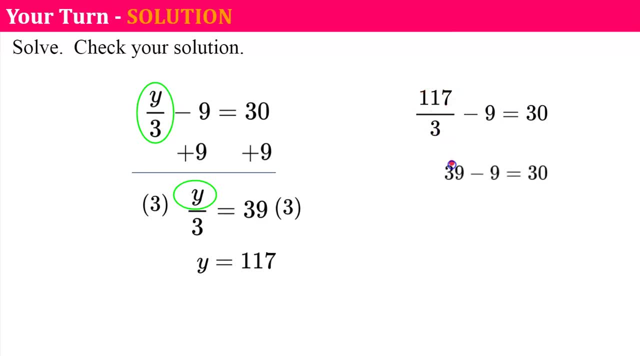 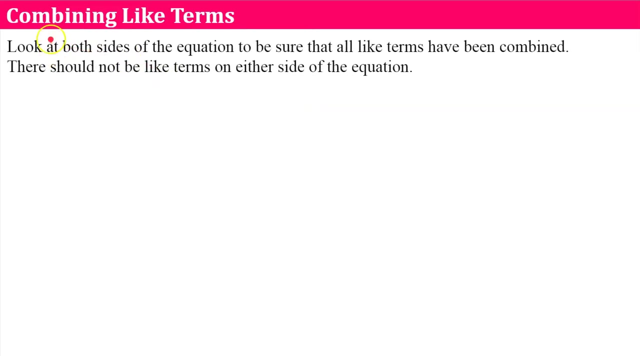 117 divided by 3 is 39.. 39 subtract 9 is 30, and it checks. Now let's talk about combining like terms. When we think about combining like terms, we want to look at both sides of the equation to be sure that all like terms have been combined. 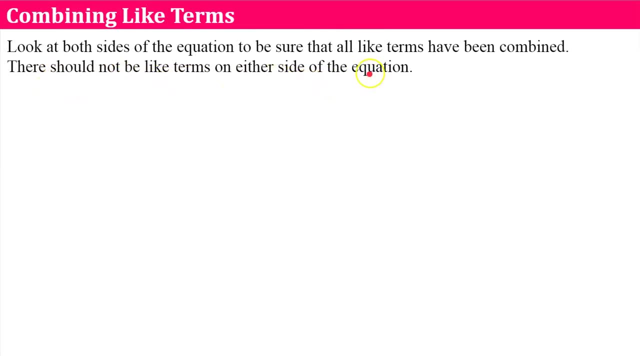 There should not be like terms on either side of the equation. Here's an example of when you would need to combine like terms. So the first thing I want to do is look for the variable term, and when I do this, I realize I have two variable terms on the left side. 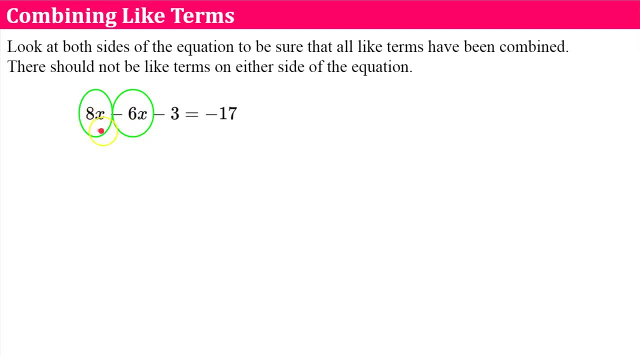 So we need to combine those, because they're like terms. They both have an x. We get to add them together or subtract. in this case, 8x subtract 6x is 2x, And then we still have the subtract 3,. 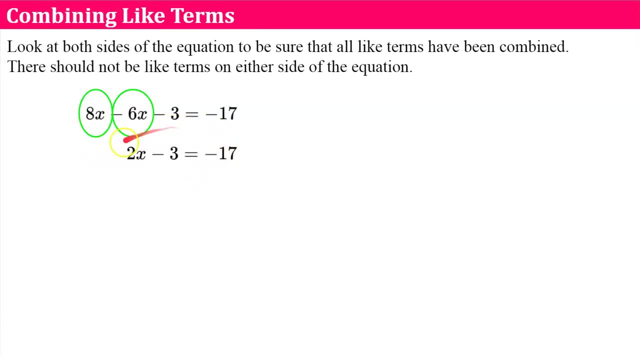 equals negative 17.. Now you can see we're back to our two-step equation. So we look for our variable term and it's being subtracted by 3.. The inverse of subtract 3 is to add 3 to each side of the equation. Again, this is 0, leaving me 2x and negative. 17 plus 3 is negative 14.. 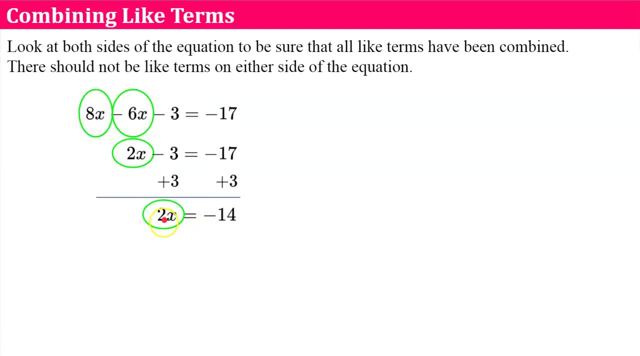 Looking at that variable term, I need to clear the coefficient. Right now, the x is being multiplied by the coefficient 2.. So the inverse is to divide both sides by 2.. 2 divided by 2 is 1, leaving me x Negative. 14 divided by 2 is negative 7.. And don't forget that big question. 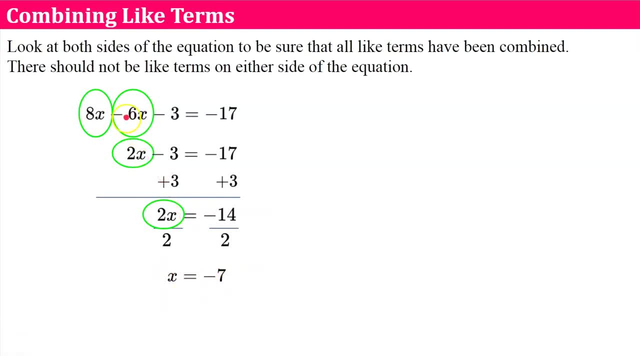 how do I know? if I'm correct, We're going to go back up to our original equation and replace the x's with negative 7.. 8 times negative 7, subtract 6 times negative 7, subtract 3, will equal negative 17,. if I've correctly solved, 8 times negative, 7 is negative. 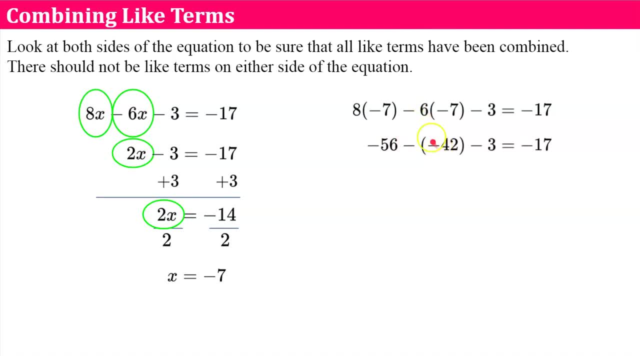 56. Subtract 6 times negative 7, negative 42. Subtract 3, and we should get negative 17.. So over here I've negative 56. add the opposite, negative 56 and 42 is gonna give me 14. 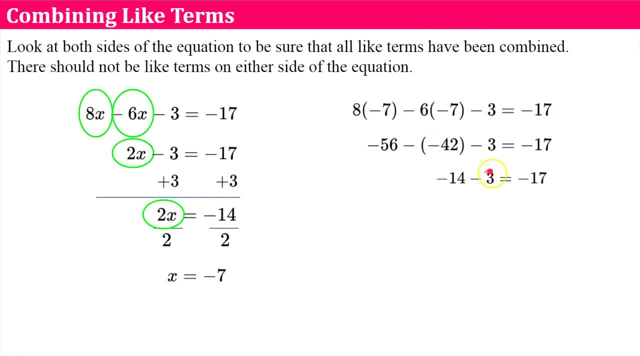 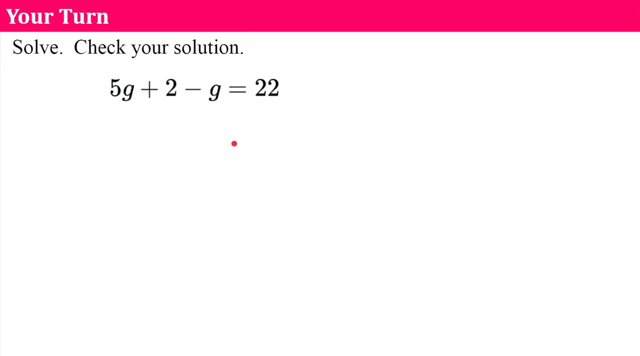 negative 14, negative 14. add the opposite: negative 14 and negative 3 are negative 17 and it checks your turn. I would like you to solve, check your solution, go ahead and pause and come back when you're done. welcome back, so I hope the 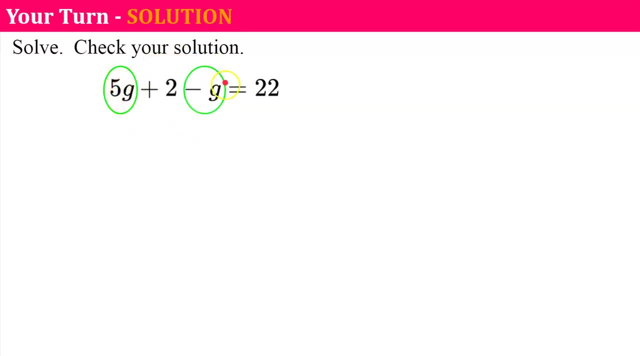 first thing you did was to identify where your variables are, and we have two. we're going to combine those first. 5 G subtract G is 4 G and I still have my add 2. now I'm going to identify that my variable term 4 G is being added by 2. 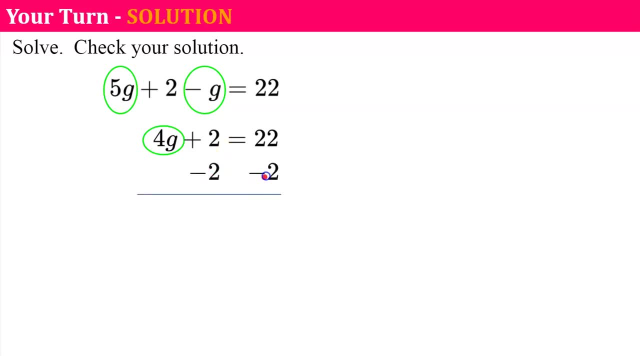 the inverse of add 2 is to subtract 2, and remember you must do that to both sides, leaving you 4. G equals 20. now my variable term is being multiplied by 4 and the inverse of that is to divide both sides by 4, leaving me G equals 5. let's check 5 times our solution of 5. 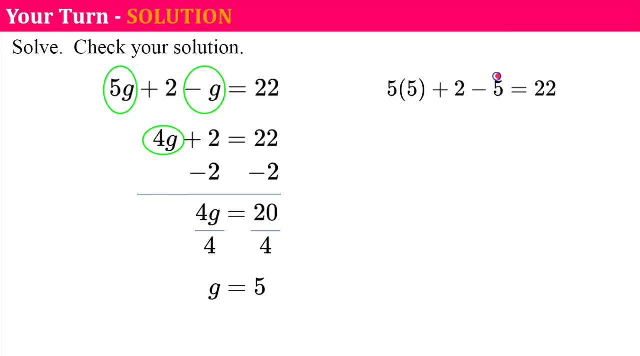 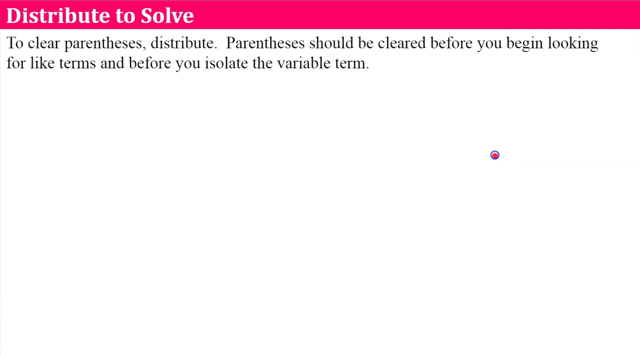 plus 2 subtract our solution of 5. 5 times 5 is 25 and 2 subtract 5 is negative. 3, 25. add negative 3 is 22 and it checks. now we're going to talk about distributing to solve. we want to clear. 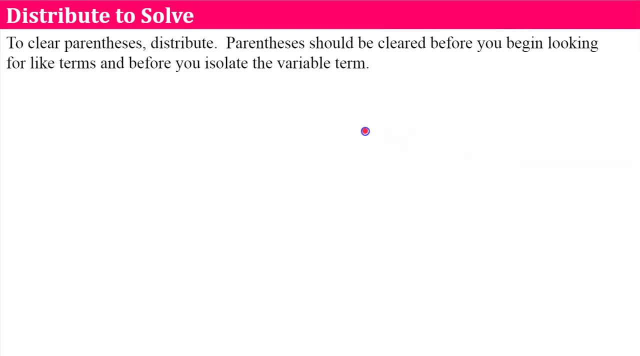 parentheses, and when you do that, you're distributing. parentheses should be cleared before you begin looking for like terms and before you think about isolating the variable term. so here's an equation with parentheses. I cannot do anything until I distribute, so I'm going to multiply this negative 2. this is negative 2 with an invisible. 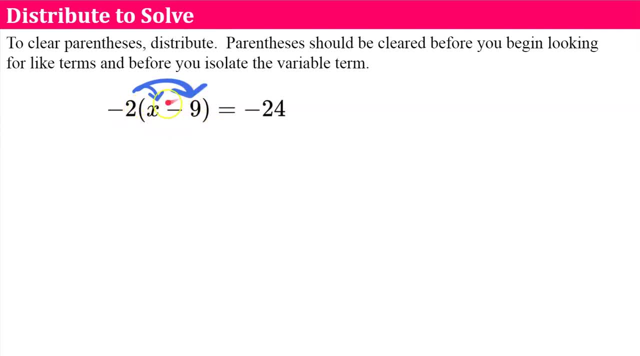 multiplication sign: times the quantity x minus 9. since X minus 9- these are not like terms. I need to distribute or think of it as sharing. so negative 2 times X is times negative, 9 is positive 18.. Now I look for my variable term. It's being added by 18.. 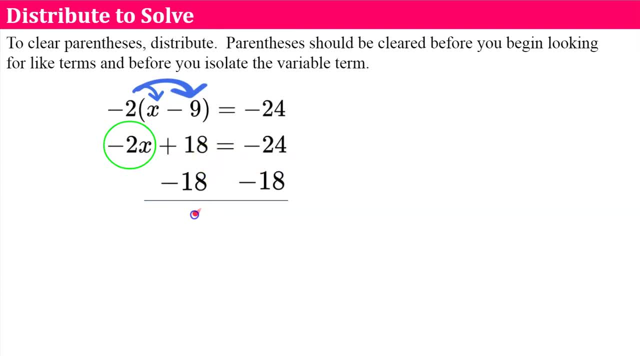 The inverse is to subtract 18 from both sides, leaving me negative 2x equals negative 42. Again my variable term. I need to clear that coefficient. It's being multiplied by negative 2.. The inverse is to divide both sides by negative 2, and I get a solution of x equals positive 21.. 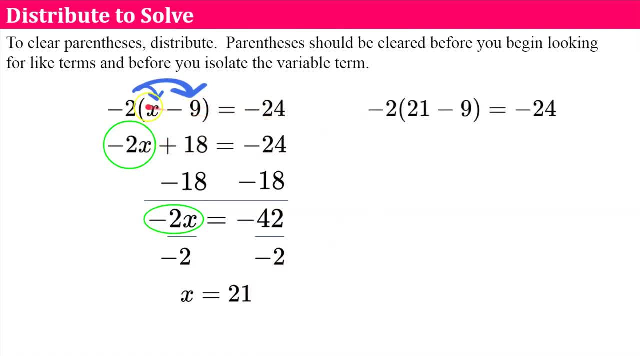 Coming back up to our original equation, we're going to check, We're going to replace x with our solution of 21.. 21 subtract 9 is 12.. 12 times negative, 2 is negative 24, and it checks. 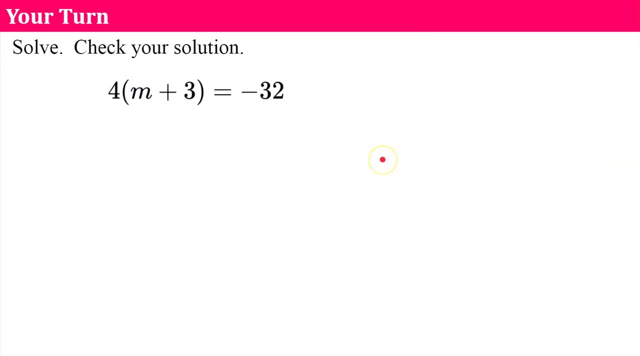 Your turn. I'd like you to pause, solve and check. Come back when you're ready, Welcome back. So our first step is to distribute. We're going to do 4 multiplied by m and 4 multiplied by 3,. 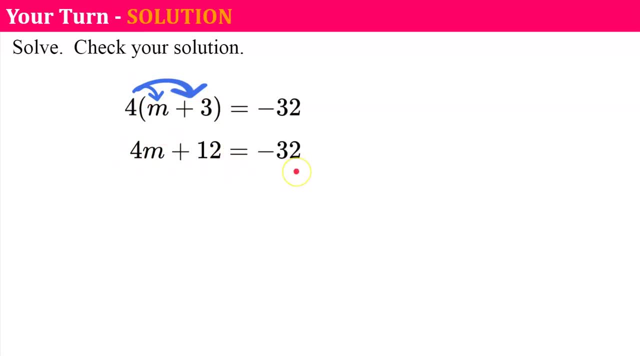 which gives us 4m plus 12 equals negative 32.. Find our variable term. We're going to do the inverse and subtract 12 from both sides Gives us 4m equals negative 32.. We're going to clear the coefficient by doing the inverse and divide by 4, and m equals negative 11.. 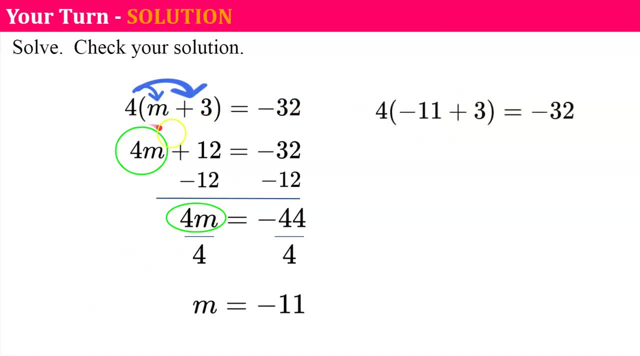 Let's check our solution. We're going to replace m with negative 11.. Negative 11 plus 3 is negative 8.. 4 multiplied by negative 8 is negative 32, and it checks Your turn. Let's see if you can put together everything we talked about in this video. 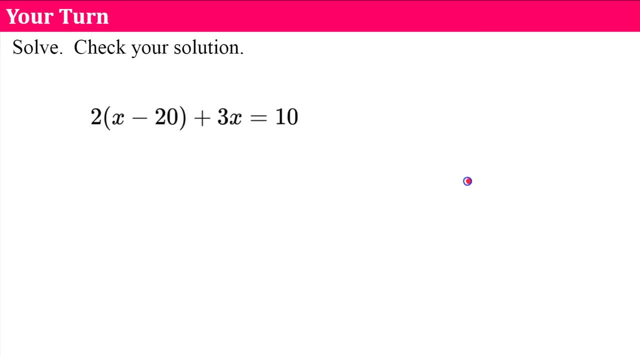 I'd like you to pause, solve, check and return. when you're done, Welcome back. So this was a little bit tricky. You had to put a few things into place that we've talked about. First thing you want to do is clear the parentheses.